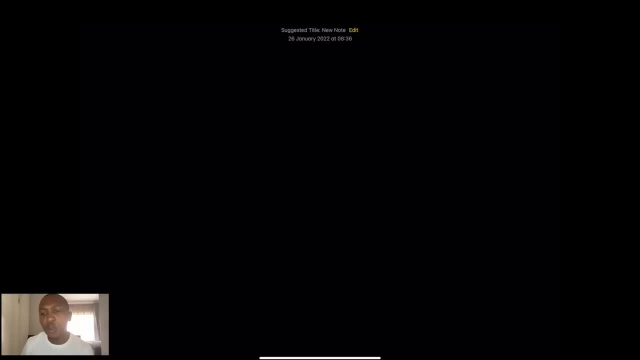 this is where you are constantly adding, you know, a number, or subtracting a number, whichever one you might, whichever way you might want to look at it, But this time around we are looking at, you know, if a sequence say, for instance, let's take 139.. Okay, let's take. 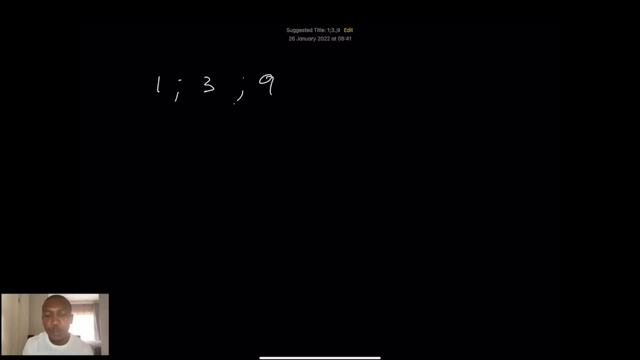 that as an example. So clearly, if you took the difference between three and one, that would give us two, And the difference between nine and three, definitely that would give us six. So clearly what's happening here is that you are not, you cannot be adding, you are not adding a constant. 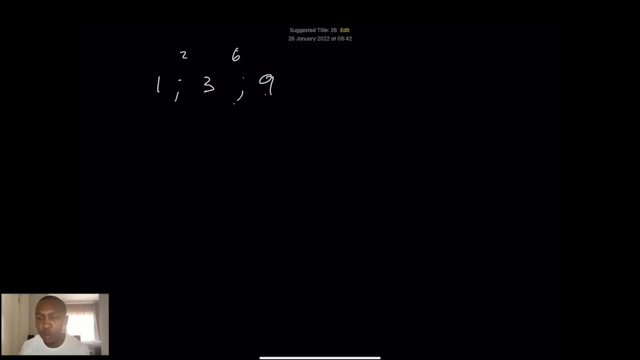 number. Okay, so it is not an arithmetic sequence, Right? However, if now I want to look at what is happening here, between one and three, so it means that one multiplied by three, it means that I multiplied by a number here. one multiplied by three gives me the second term, which is three. 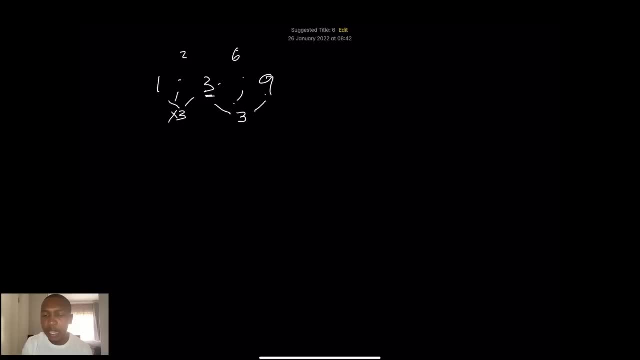 and three multiplied by another three actually gives me the third term, which is nine. Now, this time around, we are talking about a common ratio. it means that you are multiplying by a constant. Okay, So now the formula for a, a geometric sequence. we say, okay, I'm not going. 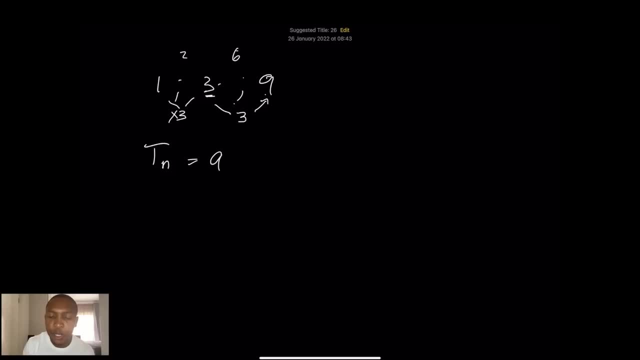 to spend much time deriving it. So we say we simply use a r to the n minus one, And remember what we said is that a is the first term, So this would be the first term of our sequence. Okay, First term. sorry about that. Okay, And r is what we call the common ratio. Okay, So that. 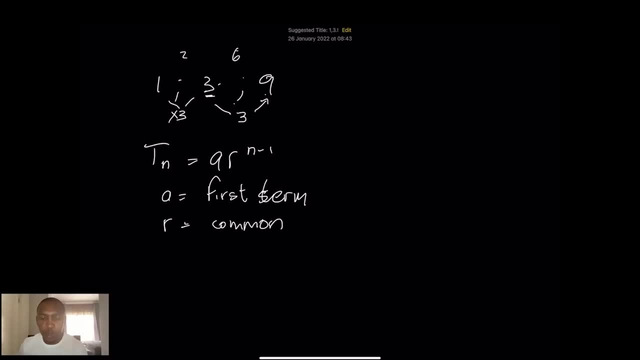 is our common ratio. Now, what we're going to do is just to look at how- how to apply. In fact, let's take the very sequence that we have there. Let's try to find the fifth term of that sequence And let's also try to find, let's say, the 10th term. 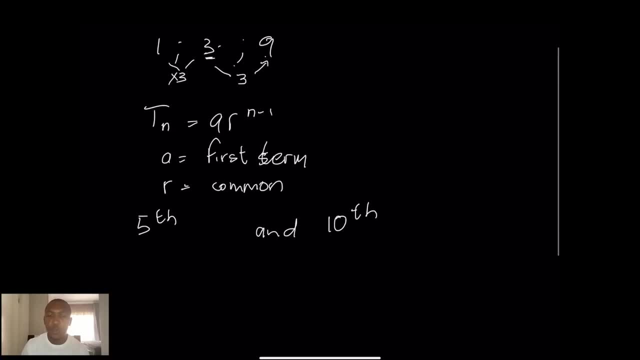 of the sequence. Okay, Right, So what you're simply going to do is we're going to identify what is our first term. So our a value is one, Okay, And our r value. we've just shown you there Now, how you work out the common ratio. please remember when we had the arithmetic sequence. 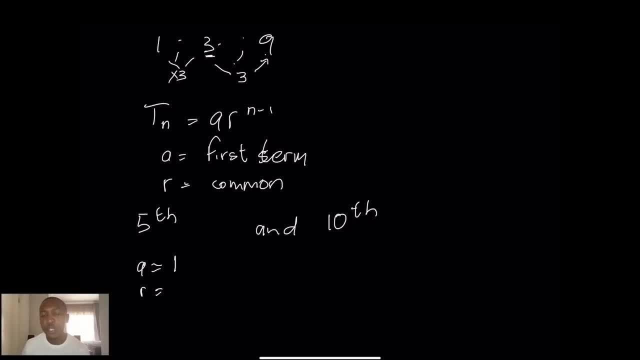 we could say: to get the common difference, you said t2 minus t1. But this time around, to get the common ratio, we'll say it's going to be t2 divided by t1. And of course you do know. 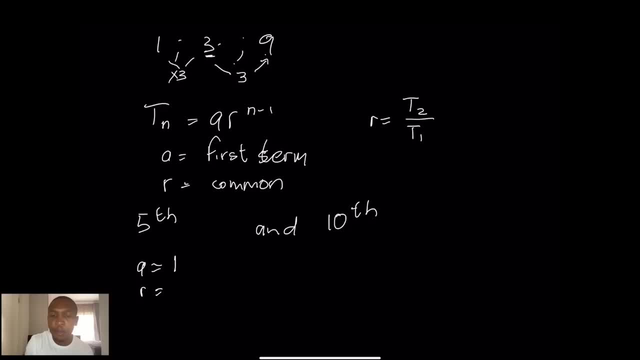 that the same thing that I did for between the second and the first term, I would do between the third and the second term. So it means that the common ratio I can simply also find by taking the third term divided by the second term. So essentially, 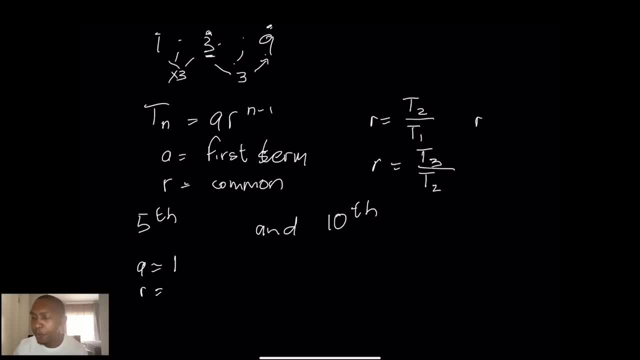 I can say to get the common ratio, Okay. I can say: well, it's going to be tn divided by tn minus one. Okay, So n would be whatever you know term it is. So if you've got the 50th term, you can say t50 divided by t49.. And that 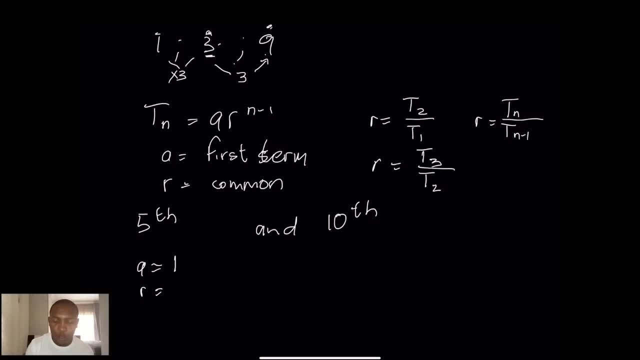 should give you the common ratio, All right. So we said our r value for the example above is three, All right. So now how do we find the fifth term? So it means that to get t5.. Okay, I will simply say it's going to be our a, So that's going to be our a. And then we're going to say, well, 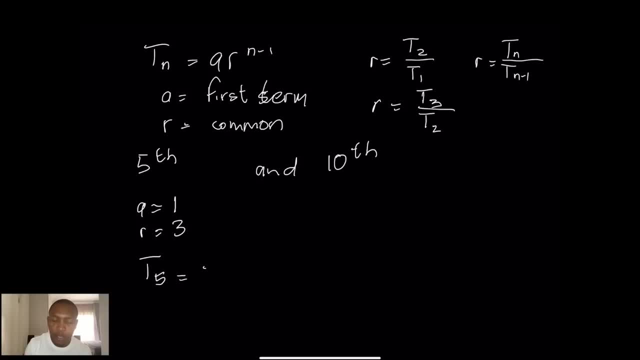 let me just write it down. So that's one multiplied by our ratio, which is three to the n minus one. So that's five minus one. Okay, So this would be our fifth term. So in this case we're going to say, okay, these are exponents now. So we're going to say: this is: 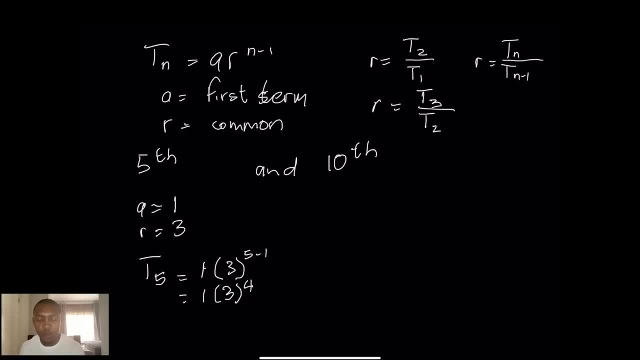 three to the power four. Okay, I'm just dragging it so that you can just simply see what I'm doing there, So that it's easy to follow on for you. Right, So to get the fifth term of our sequence, Okay, So. 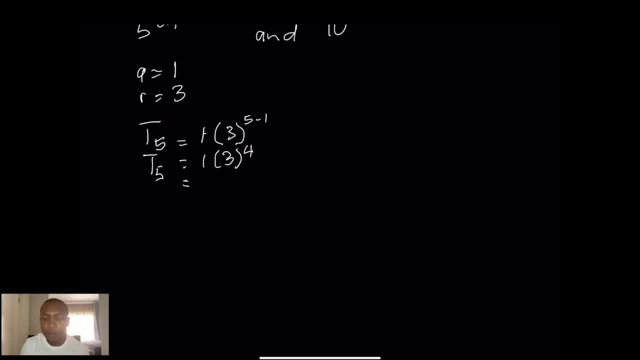 we just simply say t5.. Okay, Let's do some exponents there. So what is three to the power? four: Okay, If you note that's going to be 81, you can put that on your calculator. three: yx4. 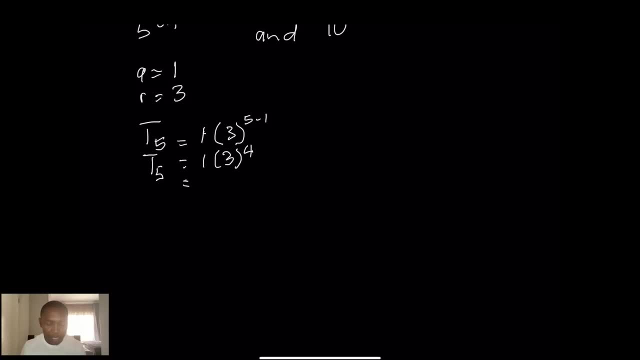 Okay, So that should give me, remember, that's three times three times three, Okay, And that should give you 81. So it means that the fifth term of the sequence should actually be 81. Okay, Right, And then if we wanted to find, we said the 10th term, I believe, So I would say t10. 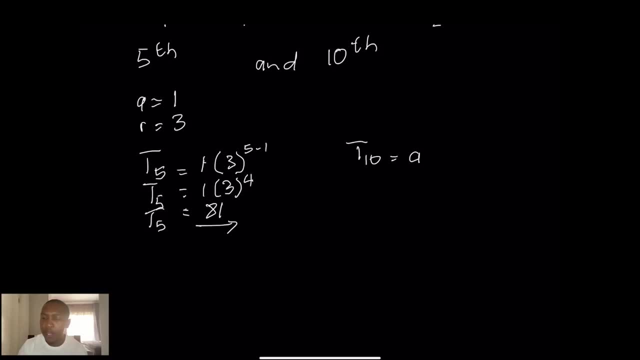 would be, again, our a value: r to the n, So that's 10 minus one. So we know that our a value in this case is one. So we know that our a value in this case is one. So we know that our a value in this. 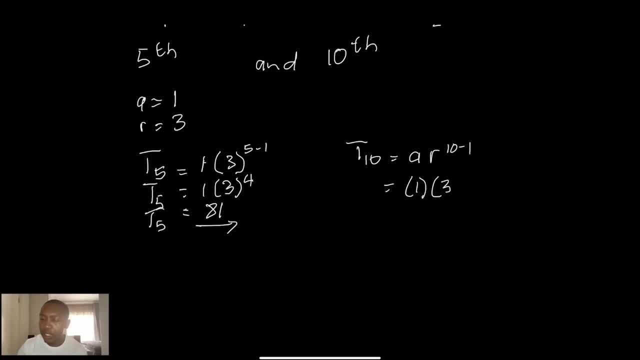 case is one: Okay, Our r value, we said it's three, And obviously to the power: nine: Okay, I wouldn't even dare attempt to put, to try and work that out on my head. So I'm going to say three to. 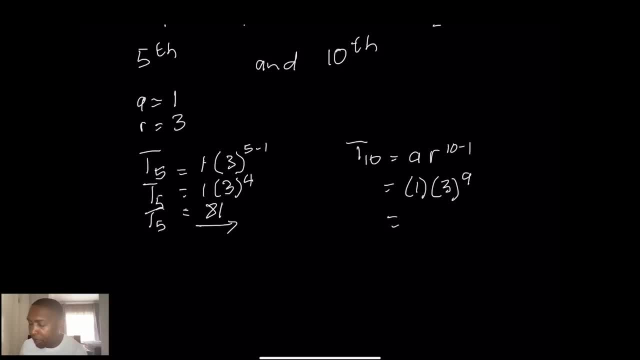 the power nine. That gives me quite a big number. and multiply that by one and 19,683.. So that would be the 10th term. Okay, So essentially that is what happens when you've got an arithmetic sequence. All right, So 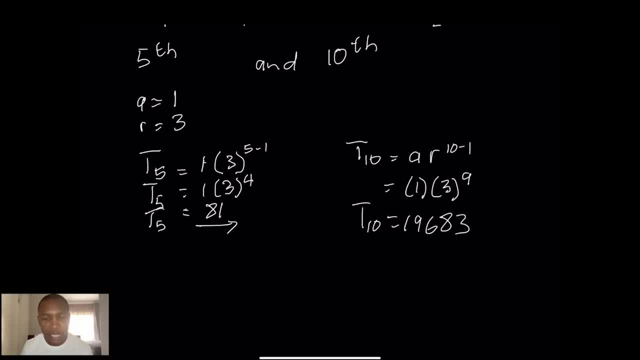 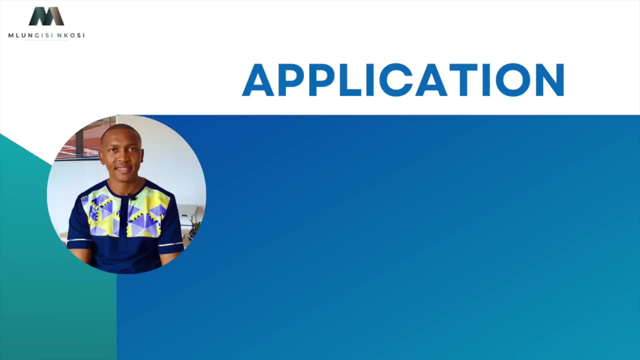 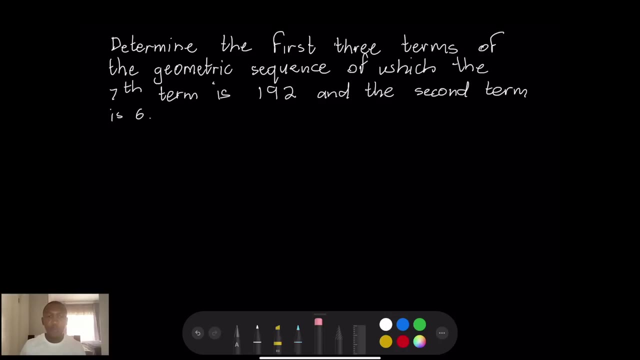 what I want to ask to do is, just to you know, take a couple of examples that we can apply this on. Okay, Once again. so let's look at this quick example. Right, They say: determine the first three terms of the equation. So let's look at the first three terms of the equation. So let's look at the. 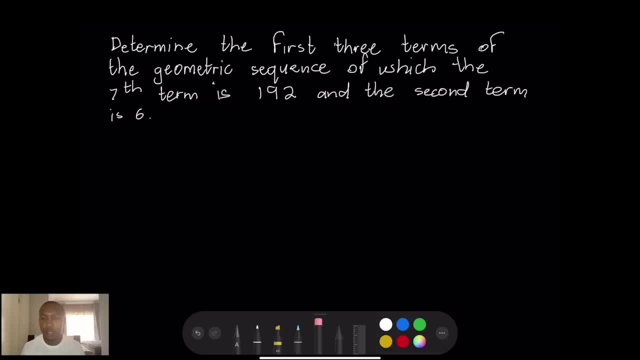 geometric sequence, of which the seventh term is 192.. And the second term is six. All right, So, first of all, we are told that it is a geometric sequence, right? So, because they've told us that it's a geometric sequence, we know the formula for a geometric sequence. However, we don't have 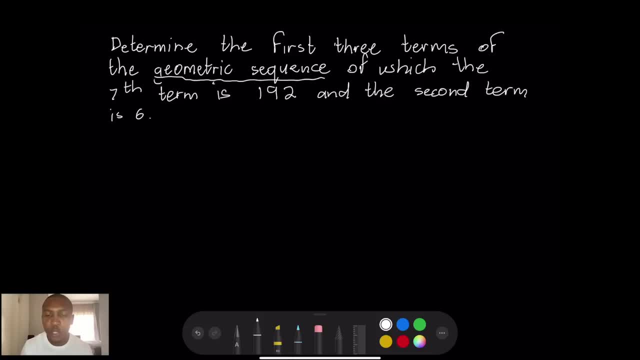 the sequence in front of us. Okay, We need to determine the first three terms. However, we do know that the formula for a geometric sequence we did say that this is a to the r multiplied by r to the power n minus one. Now, what did they give us? they gave us the second term. So it means that 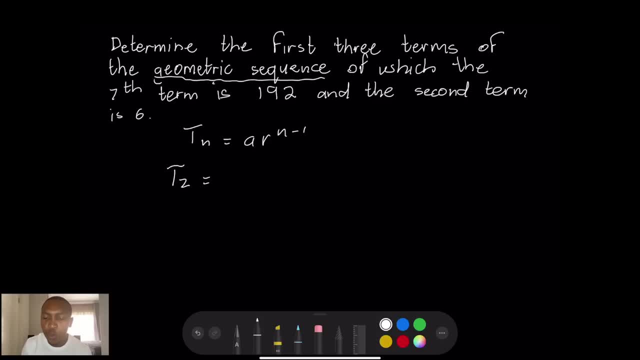 we've got t two. Okay. we don't know what the value of a is, So I'm just going to leave that as a. we don't know what the common ratio is, Okay, But we do know that n is two, So that's going to. 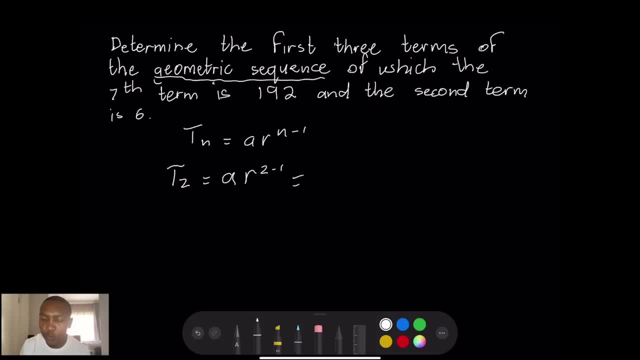 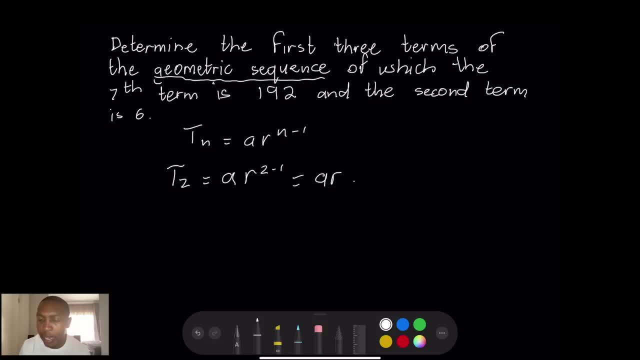 is one, So that will be r to the power one And this is equal to. if you note, there we said it's equal to six, Okay, Right, So now for t six. they said the Yeah, the seven terms. sorry about that. 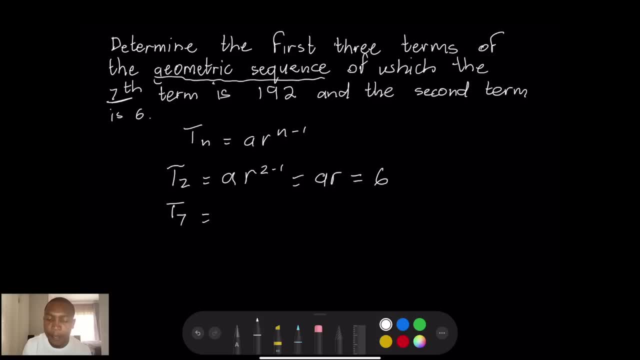 So the seven terms, so t, seven again. we know would have said a, again r, but we don't know what the value of r is. So this is going to be seven minus one, which is obviously six. So that's going to be a r to the power six And this: 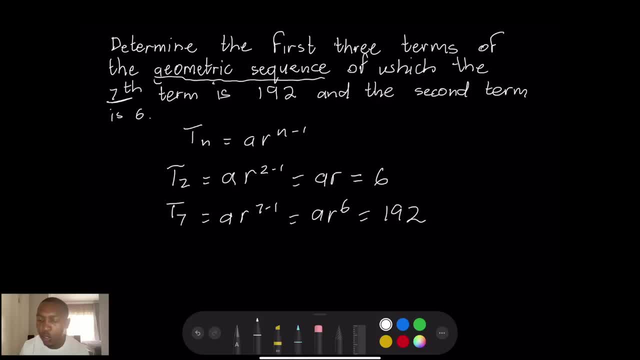 is equal to 192.. Now, let's do this. Let's say this is our first equation, Okay, and let's say this is equation number two, Right? So we've got two equations that are going to be equal to a r to the power six, So we're going to be able to solve these two equations, Okay. so what I'm going? 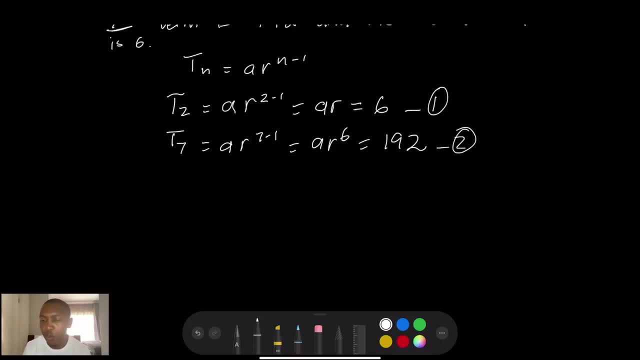 to do is I'm going to set up these equations in such a way that I can be able to eliminate at least one of the variables, And the easiest way to do that is that I'm simply going to take equation two divided by equation one, if you'll notice that. So what we're going to have is on equation. 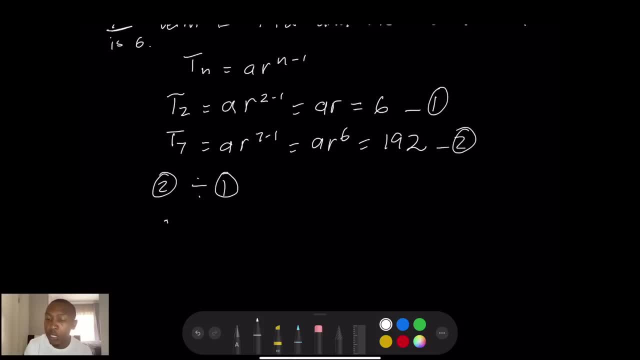 two. we've got a r equation, Yeah, equation two: Yes, we've got a r to the power six, Okay, Which is equal to 192.. And I'm going to divide the left hand side, divided by equation one, which is a to the power r, And we said this is, of course, if the left hand sides are divided. 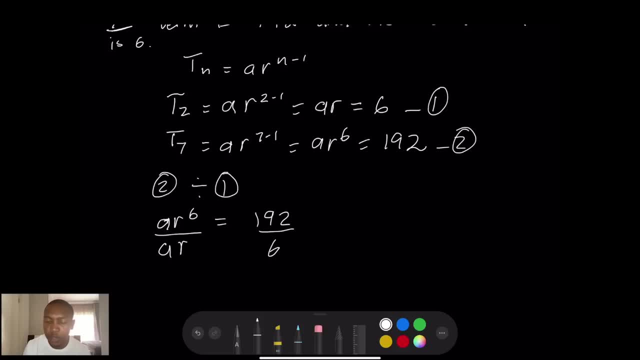 so are the right hand side. whatever I do on the left, I do on the right hand side. Okay, so what that does is that I'm dividing two things there. So it cancels out the A's, And now exponentially. what do I have? I've got r to the power six. 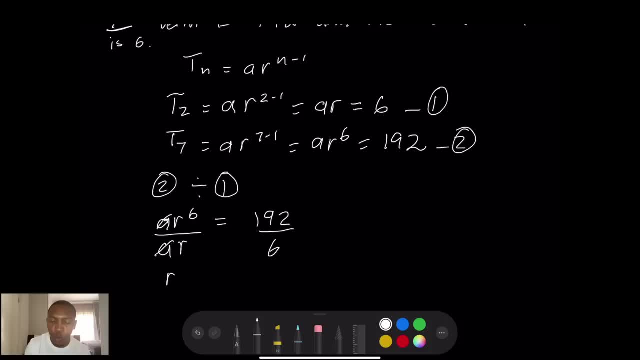 divided by r to the power one. you know the laws of exponents. Okay, for those of you who haven't done that, of course I haven't covered it in this channel as yet, But I will get to it. So what we simply are going to have is that we're going to end up with r to the power. 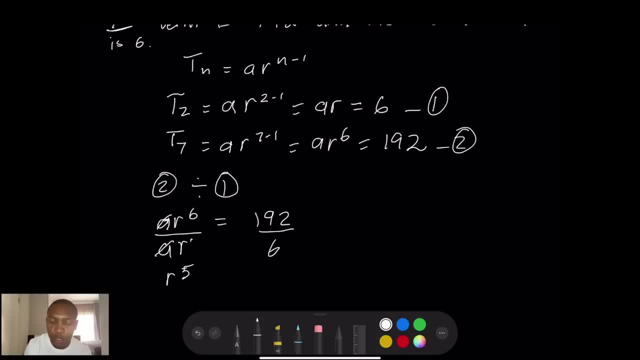 five, because we have this to the power one. So we know the laws of exponents. that's going to be six minus one. Okay, I'm trying to write as neatly as possible. Okay, so I'm going to have six minus one And let's see what's a what's 196.. So 192. 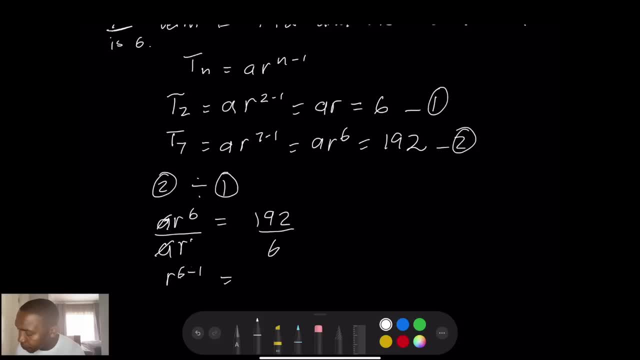 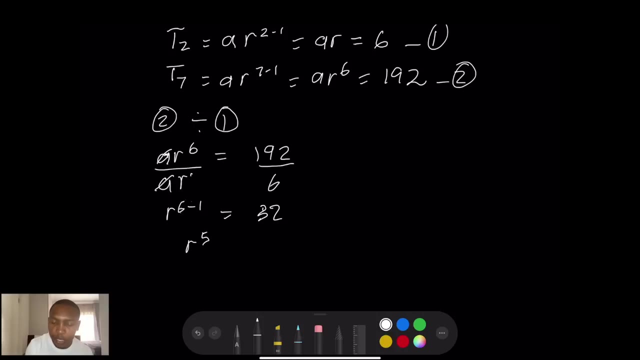 divided by six. Okay, I've got my calculator right in front of me. Okay, and it's giving me an answer of 32.. Okay, So now I know that it means r to the power five is equal to 32.. Okay, so I am going to take the cubic root of that. All you can just simply do. 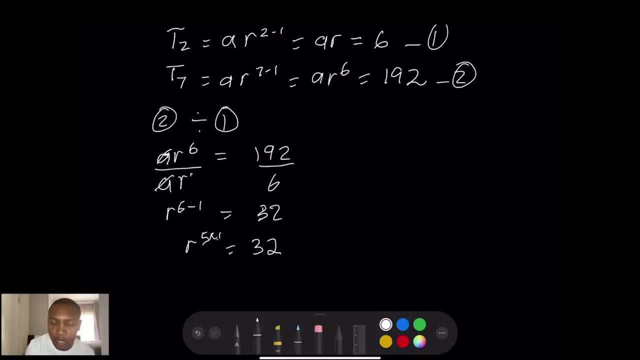 is just say multiplying that by one over five. But remember, what you do on the left hand side, you do on the right. so that's to the power: one over five. Okay, so I've got r Now, if you think. 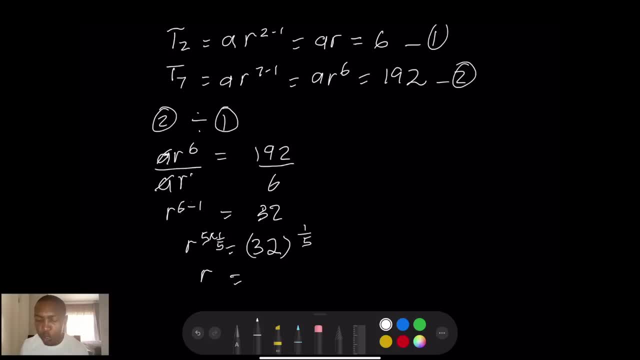 about 32,. this is the same as two to the power five. So one thing about the laws of exponents: whenever you've got exponents, what you try and do is that you break them down into prime factors, right? So 32, how can I break down 32 into a prime factor? I realized that. 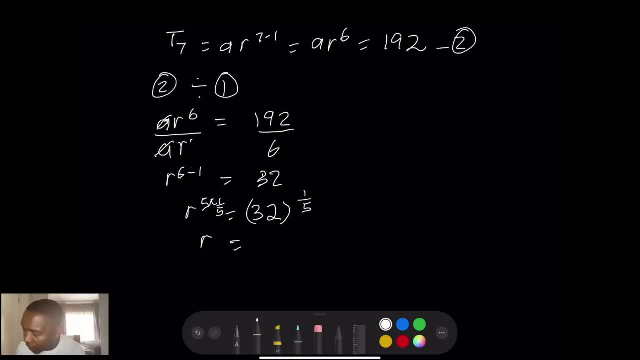 you can just put it in your calculator, right, Let's do exactly that As 32.. And that's going to be one over five And I get an answer of two. Okay, So it means that our constant or common ratio is two. Right now we need to go back and get or determine the value. Okay, we need to go. 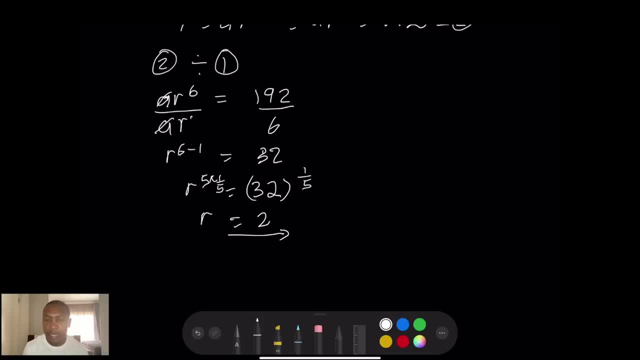 and determine the value of a. So we can now substitute the common ratio, which is r is equal to two, into, okay, let's say, equation one, so that it's easier for us. Okay, So remember, we had that for equation one, So it: 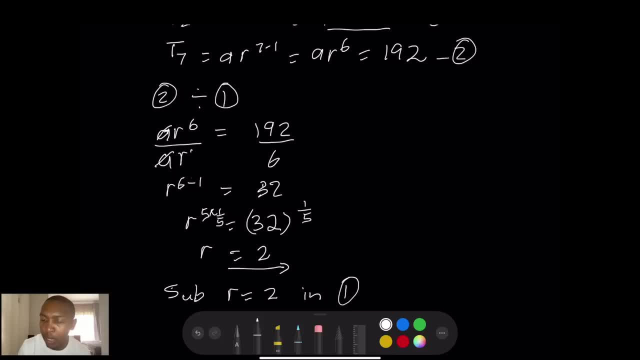 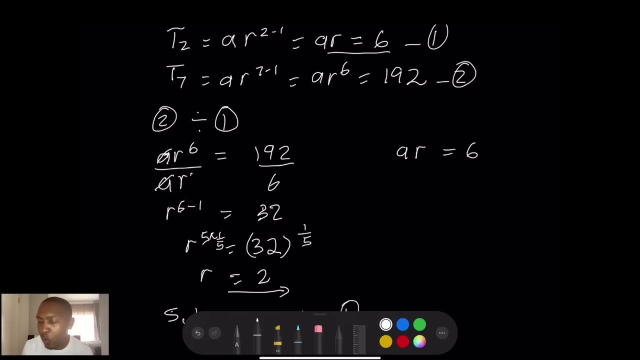 means that we're going to find our common ratio. I mean our first term. So we know that a r is equal to six. we said our first second term, rather, was six. So now we know the value of r. So we're going to say: 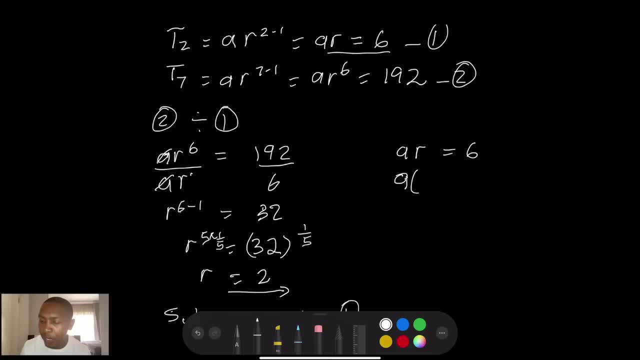 we're looking for the value of a, but our r value? we just found it to be two, And this is equal to six. So of course, we can divide both sides by. sorry, I'm already thinking about the answer in my head. So divide both sides by two, Okay? 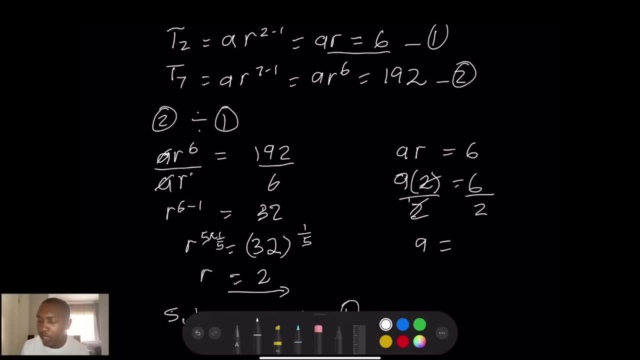 So here I just have the animator equation. this one's a little bit easier, but I'm going to continue here. So a is equal to three, six is equal to two is equal to three. Okay, so now we know that this 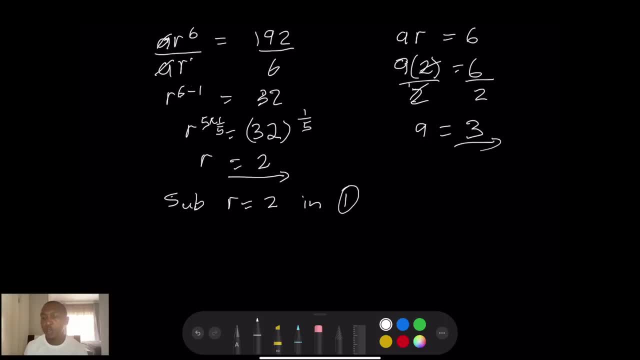 is our common ratio, right? So let's now try to find out what is our common ratio. So, to find out what this is, the first term is three, So the second term is five. Now let's try and find out what this is. So a is equal to three. six divided by two would be equal to three. So now I've got my. first term as well as my common ratio. now let's find, let's try and find out what is. what is our sequence? So we've got our first term is three. But how do we determine the second term? we simply say, to get the second term, we will go to our next equation, our index. So I'm going to go into this. 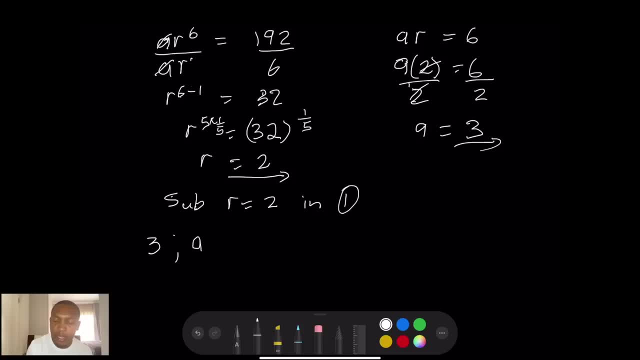 remember, i am going to say a r to the 2 minus 1 to get the third term. what do i do? it's a r to the power 3 minus 1. remember, that's constantly what you do: um with um, with geometric sequences, right? so let's do that. so this is going to be 3, that's our first term. uh, what's our a value? that's. 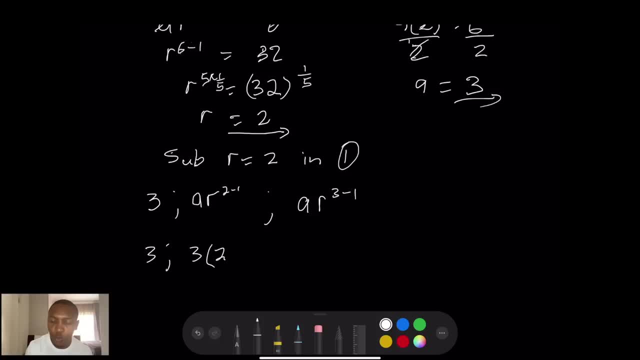 3. our r value is 2, 2 minus 1. that would give us 1. okay, and our third term, 3. that's going to be 2, and that's 3 minus 1, and that would give us 2. so let's try and get that. so that's 3. 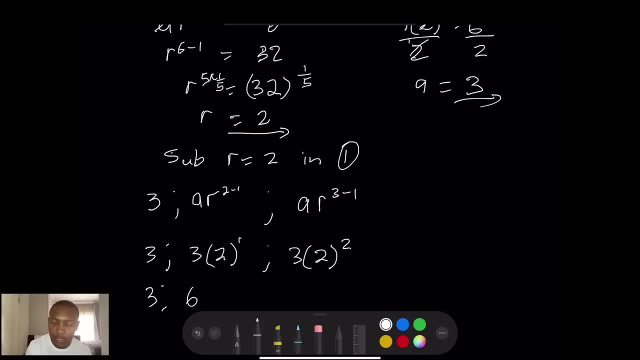 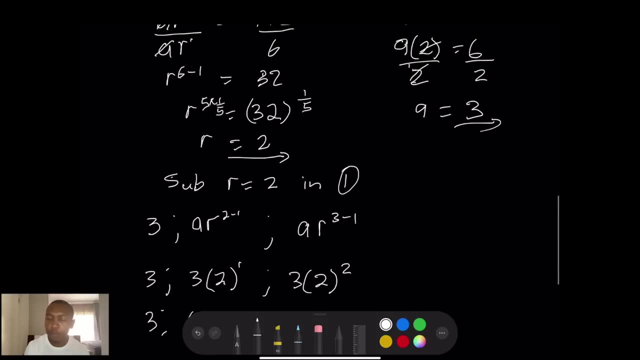 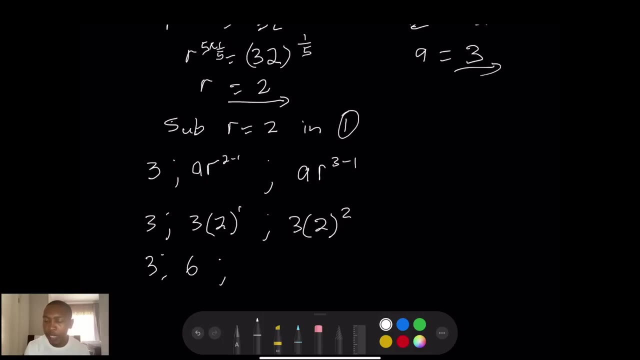 3 times 2, that would give me 6, okay, and it does concare quite well with what we found as being the second term. uh what, as we were told, right? and then, um, here we're going to start with the bracket. uh, 2 squared is 4, and 3 times 4 would actually give us um 12, okay, right. 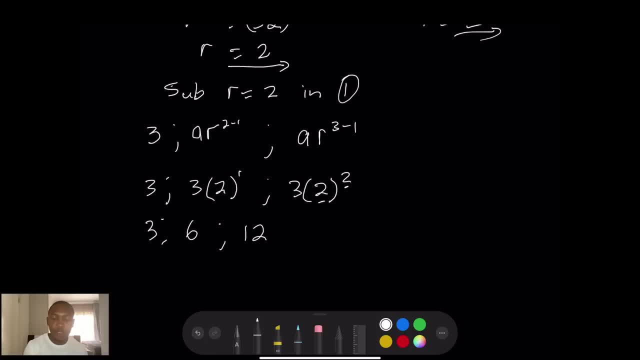 and uh, you can see that progression there. 3 times uh, 2 is 6, and 6 times 2 is 12, and of course you would have to continue and go on and on and on. okay, so that is how we would find the first 3. 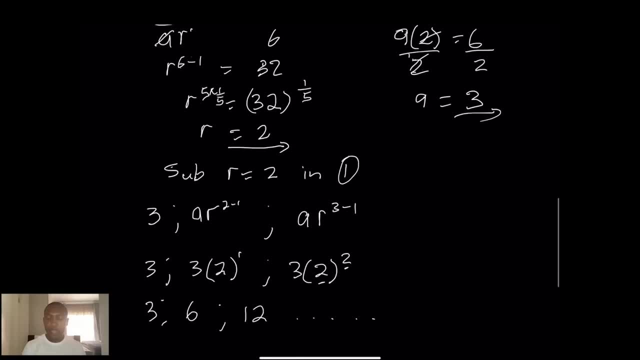 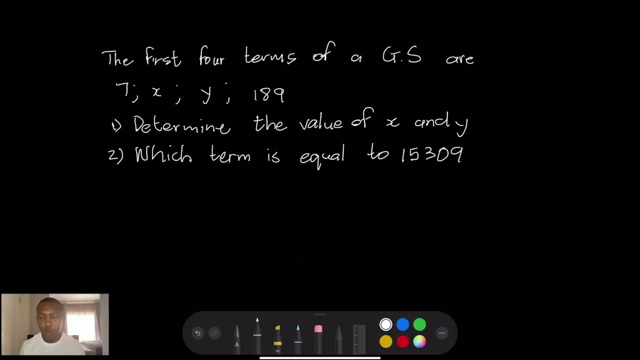 times. i hope that was helpful, right, and i want us to quickly rush into another example. okay, and we'll, um, obviously wrap up the lesson. all right, welcome again. so we are continuing. our next example. so they say: the first 4 terms of a geometric sequence are 7, x, y and 189.. Quickly, I want us to look at that. How would 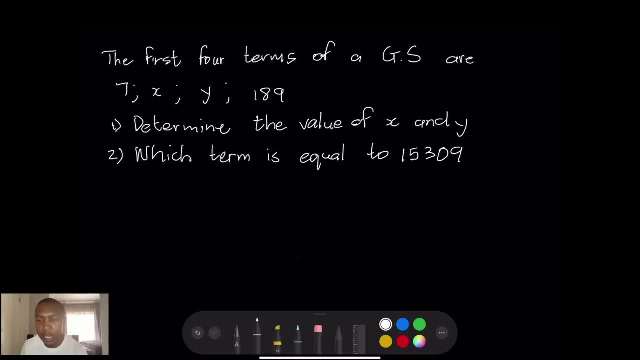 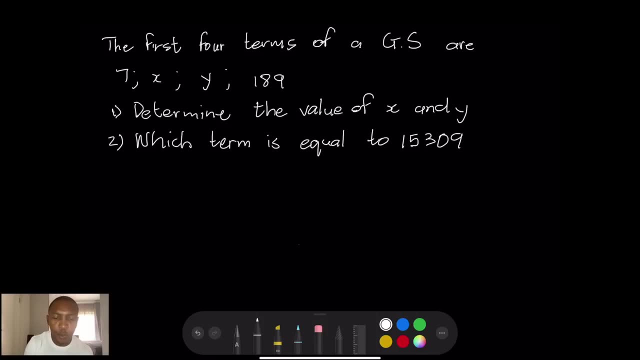 we tackle that question. They say: determine the values of x and y. Now, we don't want to overly complicate it. Now what we have there is the first term. So we already know what a is. a is equals to 7. But we don't have the common ratio. Okay, But I want you to note we already have a. 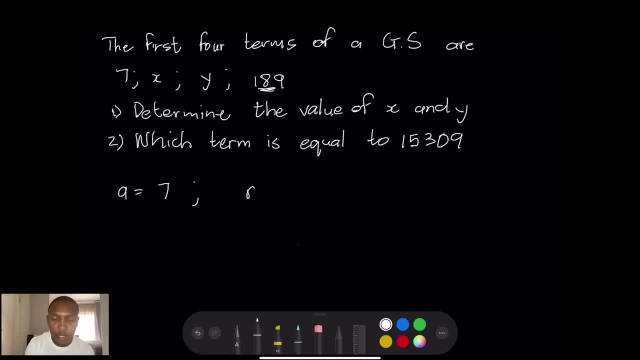 value for the fourth term. Okay, So let's take that quickly. So we know that a is 7.. But we also know t4,, which is a times r to the 3, is equal to 189.. Okay, so let's try and work that out, I know. 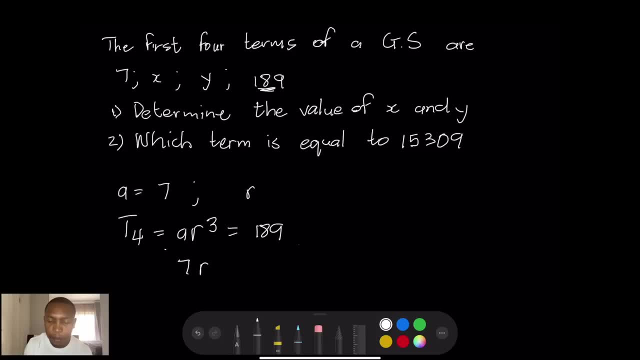 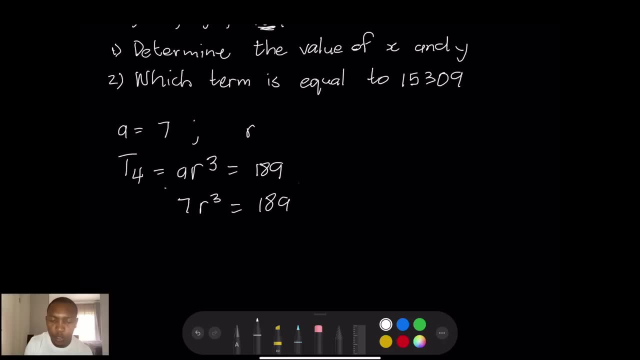 what the value of a is. that's 7.. multiplied by r to the power three, equal to 189.. Okay, let's work that out. So divide both sides by seven first. Okay, So that would be 189 divided by seven. That gives me 27 r to the power three. 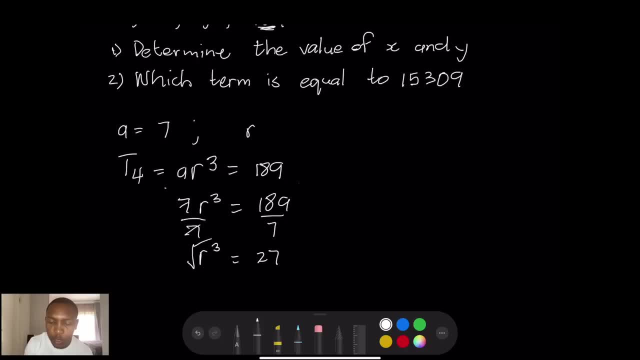 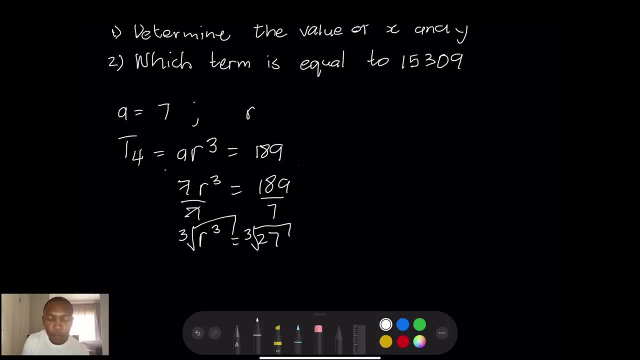 is 27.. And all we simply do is take the cube root of that. But remember what I do on the left, I do on the right. just a quick warning: If this was, we're taking the root of a- you know- often an even number. remember that the answer can. 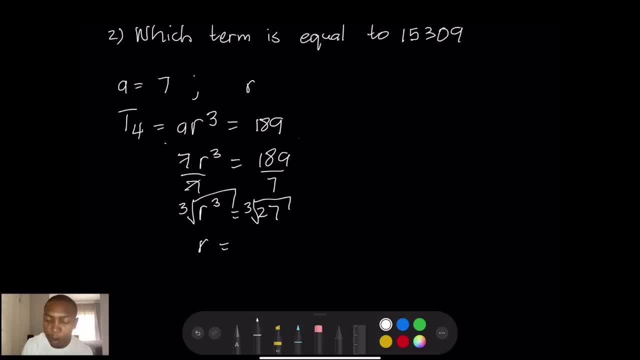 possibly be plus or minus, But because it's an odd number, we can just leave it, as you know, with a sign that it has. So in this case I get r is equal to three. So we've got now the value of a. 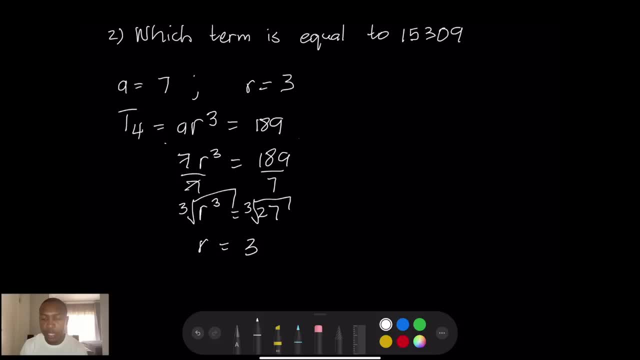 and we've got the value of r. we know that our r value is actually equal to three, right? Okay, we're first going to uh, take the root of a, So I'm going to put it over there. Let's go back to. 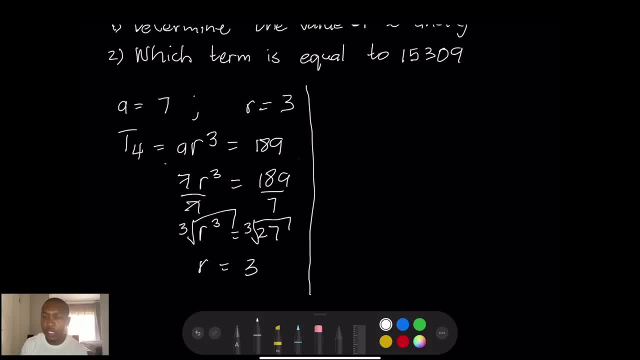 the first one. Y is equal to six. Now, I'm going to go back to the first one. So I'm going to go back to the first one. So I'm going to take the root of r. This is actually number three, right? Okay? 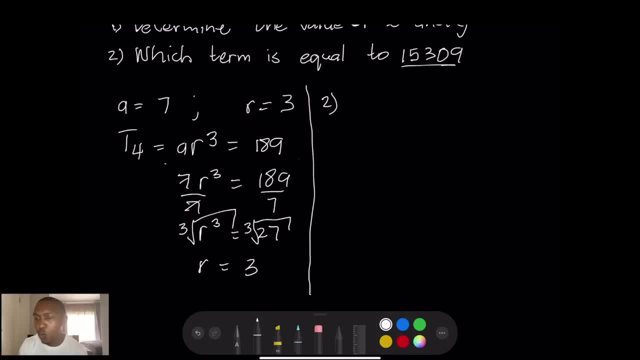 and I'm just going to add another side. So now let's do it to the right. So the first time I want to do this is to take the root of a plus r to the power three. right, Okay, and now it's. 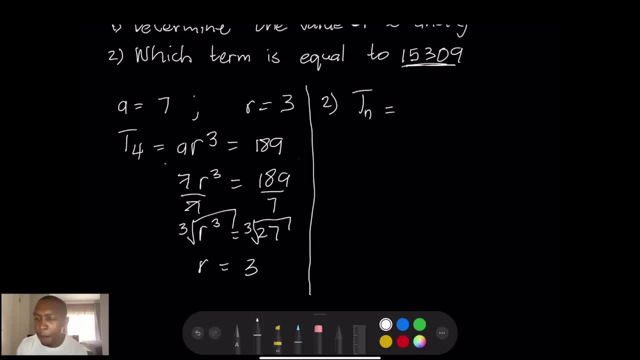 going to be 15,309, rather Okay. so let's find that out quickly If you don't mind, just going to do it just next to this here. So this is our second solution. So now we want to know which term is actually 15,309.. 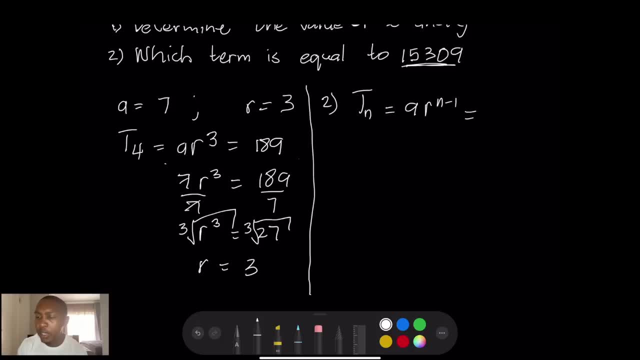 r to the power n minus 1, and this is equal to 15309. okay, so we already know two things. we know that a is 7, we know that r is 3, but this is the power n minus 1 and please, i'm just going to. 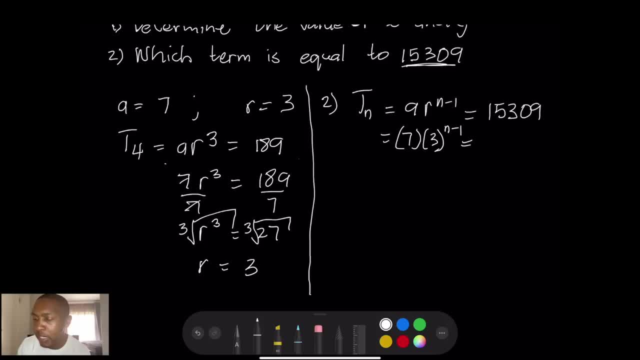 introduce something here. i know i haven't done it on the channel as yet, but i want to show you how to tackle this type of a question. okay, so, that's 309, okay, so, uh, first of all, you cannot multiply between those two because, remember, the three already has a power in it and that's power n. 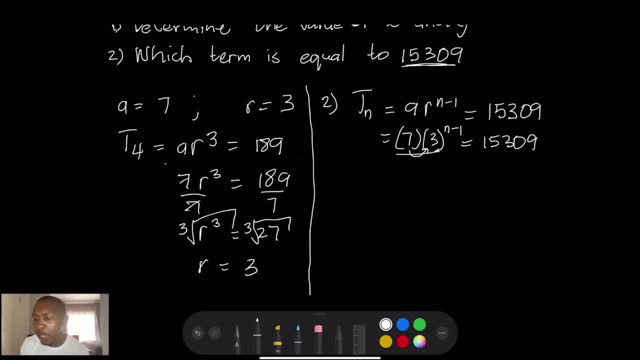 minus one. so what we can do is we can divide by seven, okay, so that we get rid of that, okay. but what we do on the left, we do on the right. so we've got three to the power. n minus one is equal to, let's see, 15309. 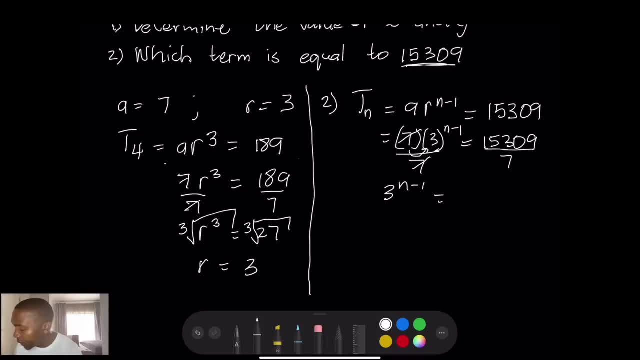 uh, divide by seven, okay, and that gives me 2187. uh, sorry, 2187. i said 89 instead, okay. um, right, so now that's 2187. okay, now, how the reason do we solve for something like this? um, i want you to please note what we can try to do. 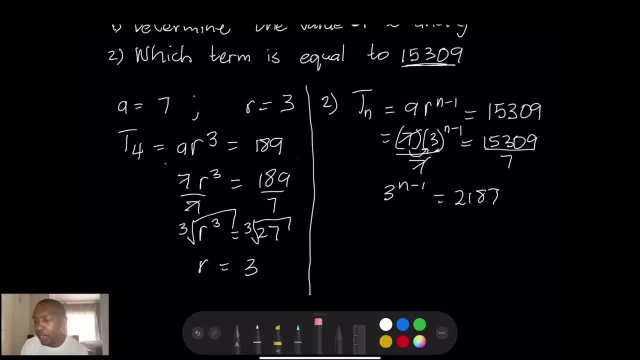 is: just try to break down that number that we have there in terms of exponents, okay, but what i would actually just uh, jump down to, you can just quickly just introduce logs, okay, it makes it simpler for you, uh, if you want to go there. so in this case, i'm. 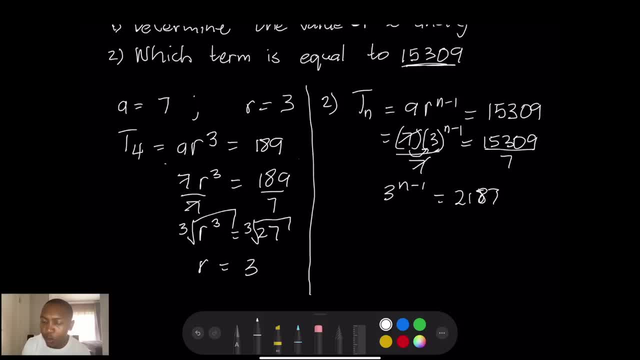 um, i'm going to do that and i'm going to say that, i'm going to do that, and i'm going to do that to introduce logs on both sides. so i'm simply going to say: well, the log of um three to the power n minus one is equal to the log of two, one, eight, seven. of course you could have, uh, worked it. 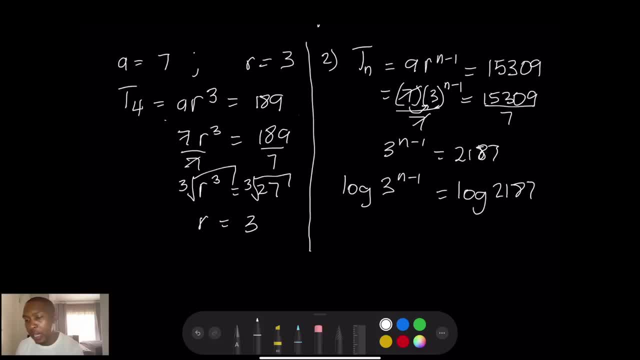 out a little bit. uh, um. yeah, there is another way in which you could have worked this out, but i'm choosing this one, okay. so now, uh, remember the law of logs. what you can do is that we've got a power there. okay. the jump down rule, okay, so we could have n minus one. uh to the log of three. okay, 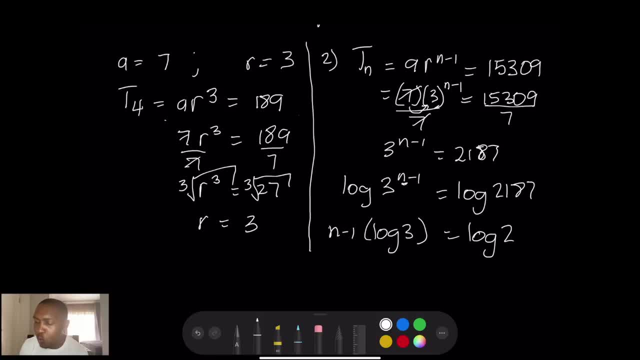 is equal to the log of two, one, eight, seven, okay, and all you simply do. we've got n minus one we can divide. uh, in fact i should have done that first. we can divide both sides by log of three, okay, so i'm going to simply say, just log three on this side, and obviously what i do on the left. 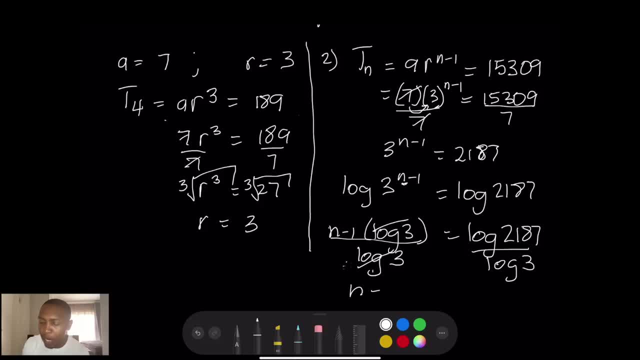 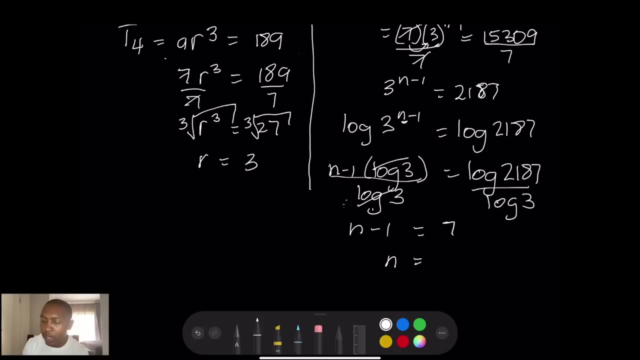 i also do on the right. so i've got n minus one is equal to. now let's take the log of that number, okay. so i'm going to say the log of two, one, eight, seven, okay, divided by the log of three, and i get seven as my answer. but remember we are looking for n, so n if i go, if i take that to the. 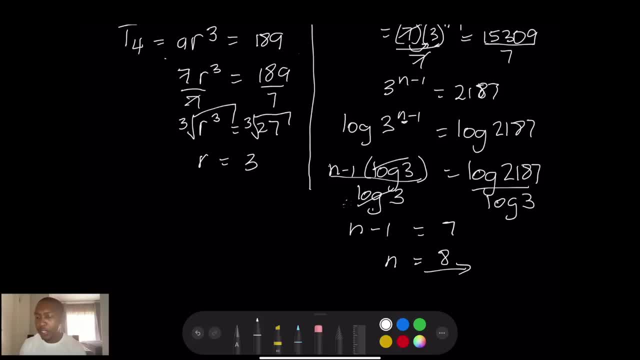 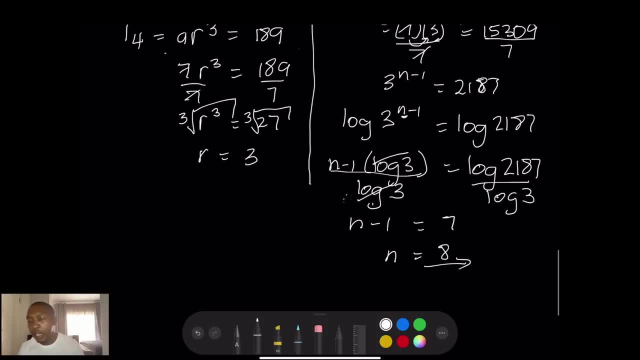 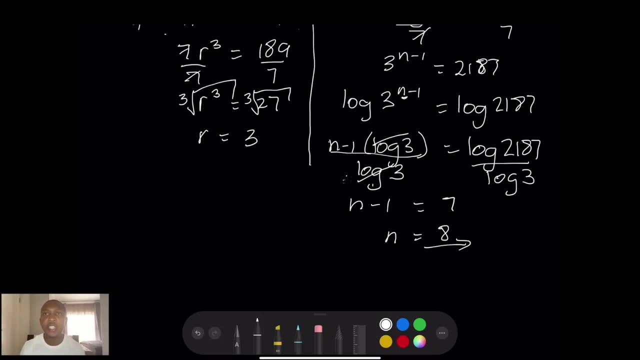 other side, n is equals to eight. it means that the eighth term would actually be the number that was given. okay, and of course, you could have worked it out in a different way, all right, but um, i i chose to take this one because it's It seems to be quicker and easier. 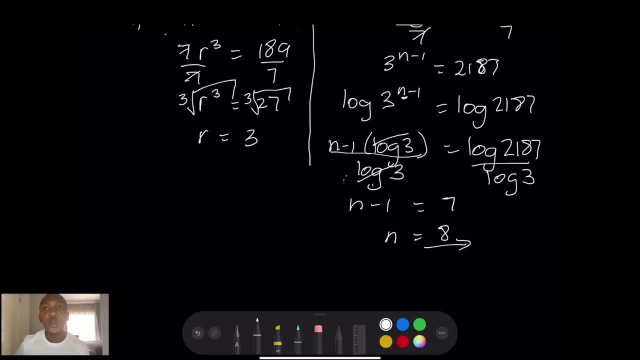 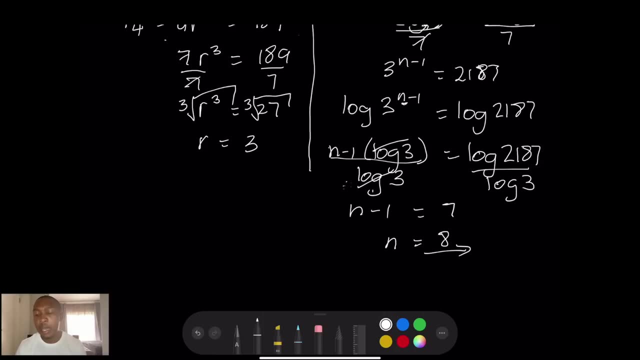 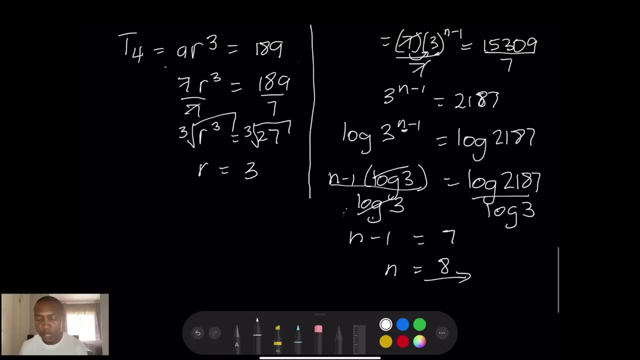 OK, so in this case, that is how the cookie crumbles when it comes to the geometric sequence. OK, we will do some past exam questions a little later on. What I do want you to do is just get yourself familiar, you know, with our manner of presentation in this particular case. 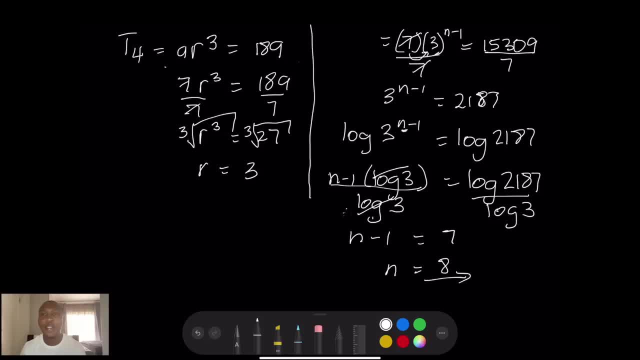 And for those of you who haven't subscribed, please just consider being part of the family And thank you so much for joining us And I'll see you guys again next time. Shab-shab.